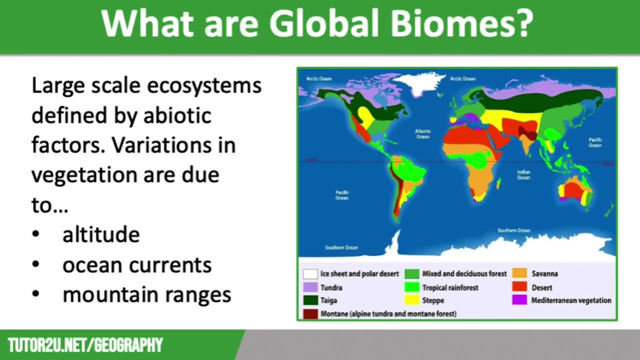 will be due to the amount of water that is in the ocean. So, for example, the altitude where, with height above sea level, This is because the air is thinner, so it cannot retain as much heat. As a result, trees are replaced by tough grasses on steep mountains. 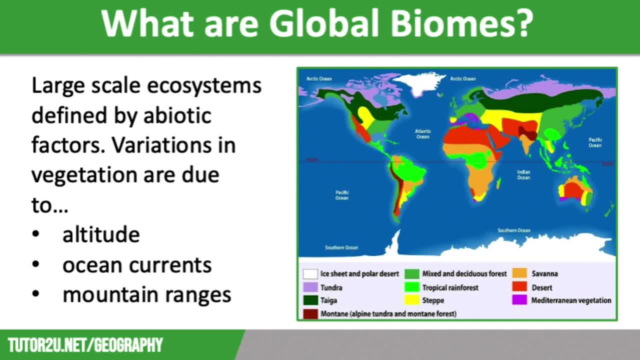 If we think about ocean currents, cold ocean currents create dry conditions because of a lack of evaporation, whereas the warm gulf stream current makes countries in western Europe warmer than they should be due to their latitude. And if we consider mountain ranges, these force air to rise. 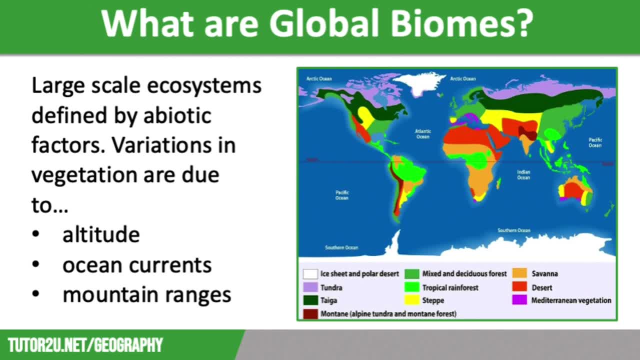 upwards, leading to a decrease in the amount of water that is in the ocean. So, for example, recording precipitation Venezuela in the Pacific Ice. dass predicted 370 Hud번 ca to relieve rainfall over mountainous areas, But this means that moisture is quickly lost. so the 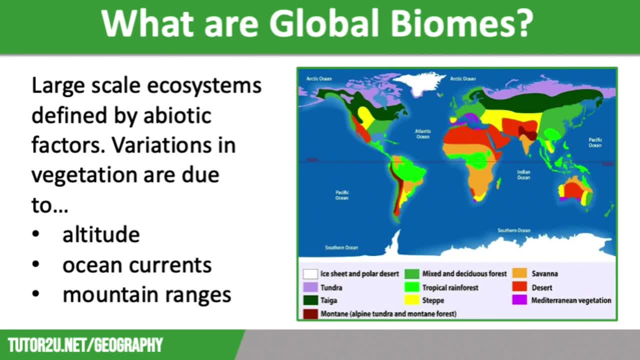 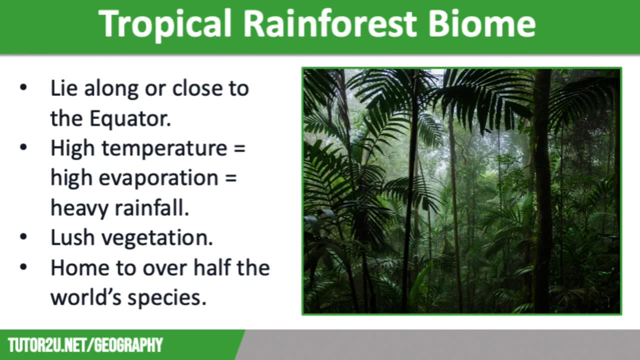 land on the other side of the mountain range is dry, Which is known as the rain shadow. We are now going to give you a quick overview of the main characteristics of the different global biomes and the salt water lactate defensures as such. So let's start off with tropical rainforests. 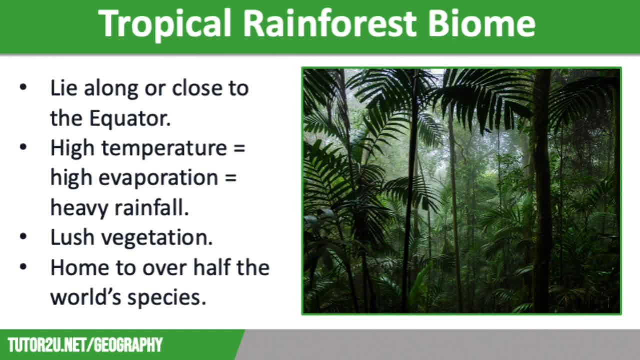 Tropical rainforests lie along or close to the equator and can be found in South America, Central Africa, Southeast Asia and Mexico. And with that being said, for your airports, explore what longeva perseguredo so called desired viewpointvos andnine thicker than you have in your countries. 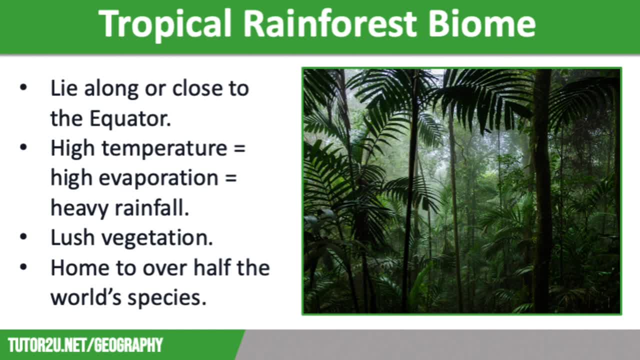 and Australia. Here, the sun's rays are concentrated, which means the high temperatures cause evaporation, and the moist air that rises leads to heavy rainfall, with very little seasonal variation. This belt of low pressure along the equator creates ideal conditions for plant growth, which is why the vegetation is so lush. Rainforests cover approximately six percent of the earth's land. 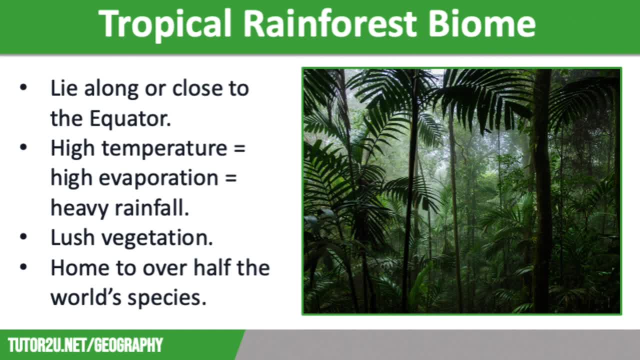 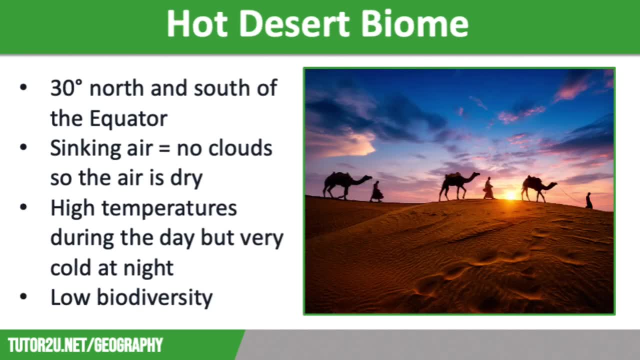 surface. however, they are home to more than 50 percent of all animal and plant species and they provide the ingredients of 25 percent of all medicines. Okay, moving on to the hot desert biome. Hot deserts lie roughly 30 degrees north and south of the equator, close to the tropics of Cancer and Capricorn. Here, the sun's rays are still very. 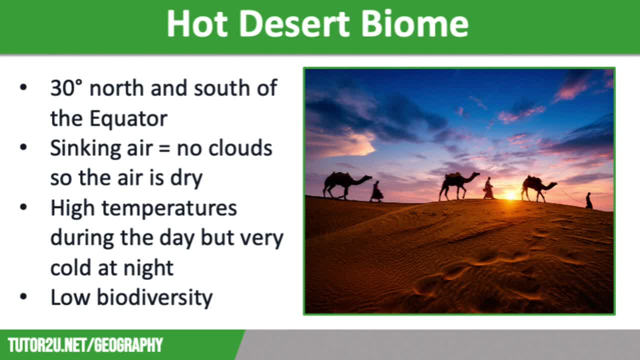 concentrated, but the air is sinking here, which means that clouds don't form, so the air is very dry, resulting in a high pressure belt and arid conditions. The lack of cloud means that the temperatures are high during the day, but they plummet overnight. The conditions in the desert biome are extremely harsh, so animals and plants have to be well adapted. 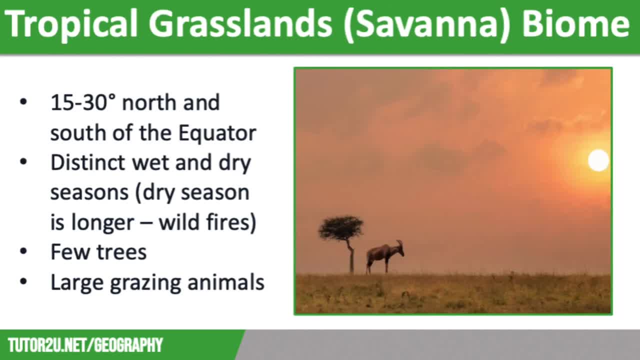 to survive. We're going to talk about the tropical grasslands biome next, which is also known as Savannah, and it may be familiar to those of you that have seen the Lion King. Savannah grasslands lie between 15 and 30 degrees north and south of the equator, between tropical rainforests. 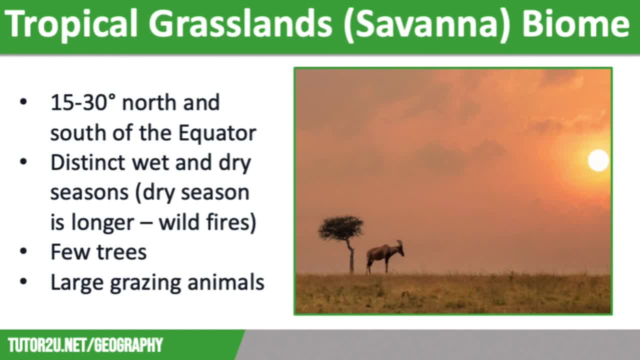 and hot deserts. This biome has distinct wet and dry seasons due to the Hadley cell. The dry season is longer and it can be extremely hot, with wildfires common, whereas the wet season can see torrential downpours and intense thunderstorms. Savannah grasslands are characterised by few trees and are home to large 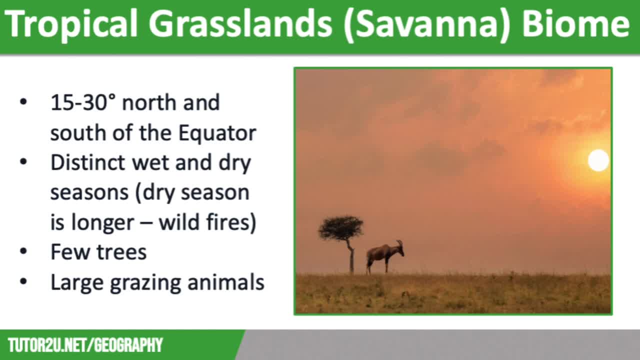 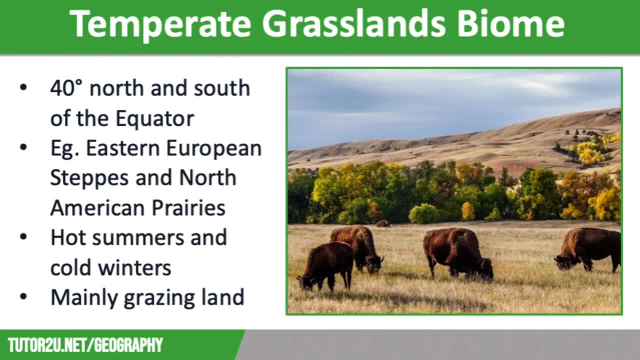 grazing animals such as giraffes, elephants and zebras, along with predators such as lions and cheetahs. Let's have a look at a different grassland biome. This time, we're going to have a look at temperate grasslands such as the eastern European steppes and the North American prairies. Temperate grasslands. 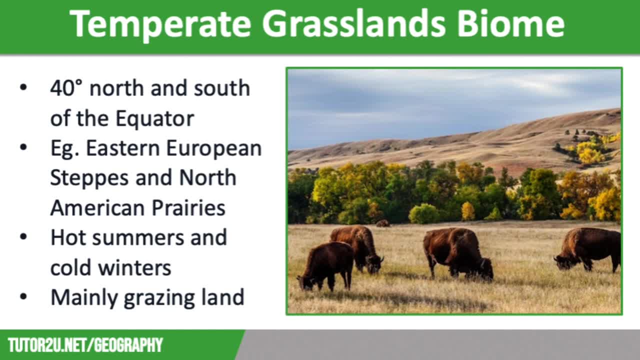 lie around 40 degrees north and south of the equator. They're in lands. they experience hot summers and cold winters, as they don't benefit from the seasonal warming and cooling effects of the sea. This biome is dominated by short, tussock and feathered grasses, and they're also 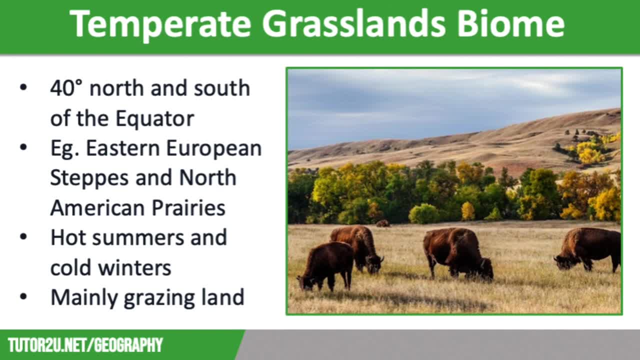 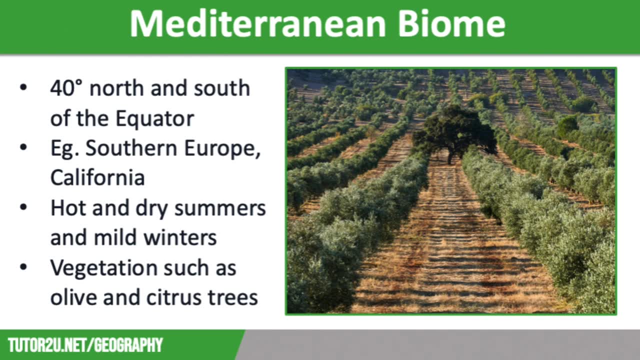 mainly used for grazing. Let's move on to the Mediterranean biome. The Mediterranean biome lies around 40 degrees north and south of the equator, in Southern Europe, California, in the USA, South Africa and Western Australia, and it is characterised by hot and dry summers and mild winters. Vegetation includes: 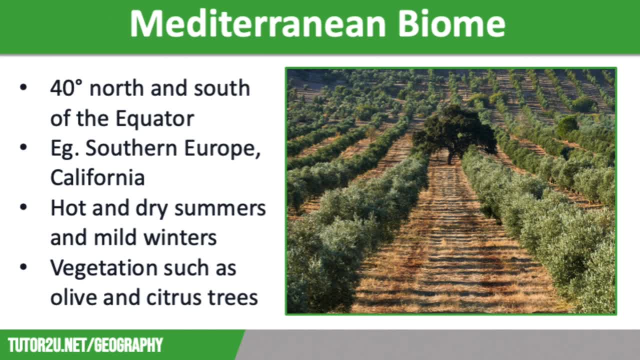 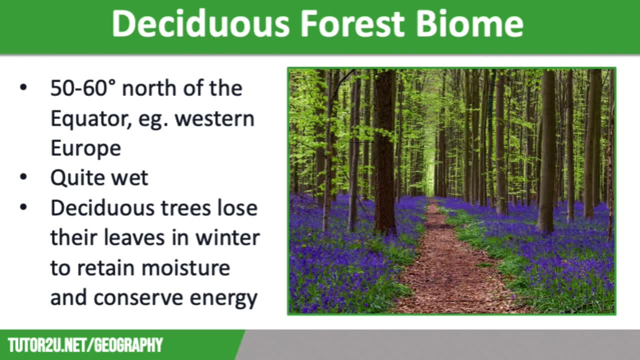 small drought resistant trees and evergreen shrubs, as well as olive trees and citrus trees. We learned about the deciduous forest in the last video on small scale ecosystems, but let's have a quick recap of this biome. Deciduous forests lie in higher latitudes, roughly between 50 and 60. 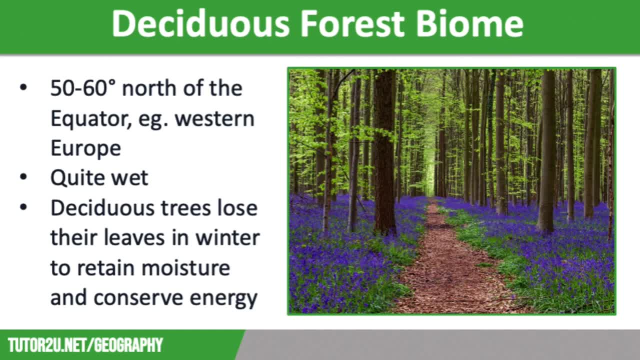 degrees north of the equator. in places such as Western Europe and North America, The climate tends to be quite wet due to the jet stream bringing in rain, and deciduous trees lose their leaves during the winter to retain their moisture. The deciduous trees are a great source of 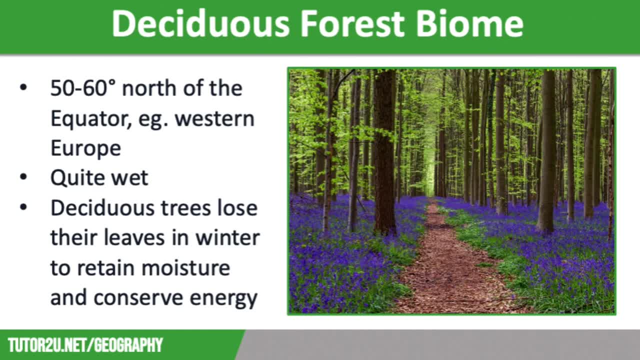 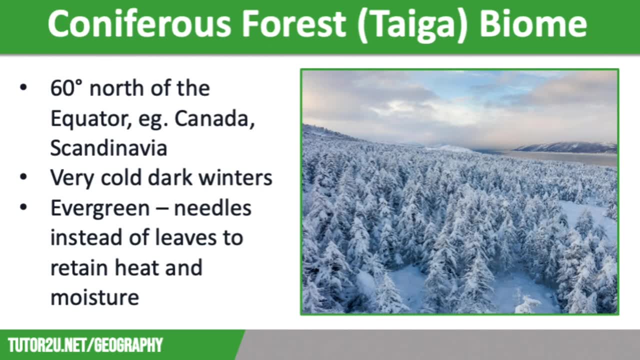 moisture, but also because there is less opportunity for photosynthesis because of the reduced sunshine. Okay, let's have a quick look at the coniferous forest biome, which is also known as the taiga. Coniferous forests are found roughly 60 degrees north of the equator, in places such as Scandinavia. 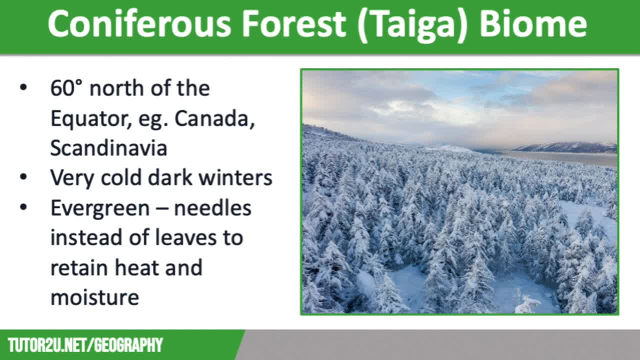 Canada and Northern Russia. Winter is bitterly cold in this biome because of the earth's tilt. there is very little sunlight for several months. Coniferous trees have needles instead of leaves, which retain heat and moisture during the cold, dark winters, and they are also evergreen, meaning that they can maximise 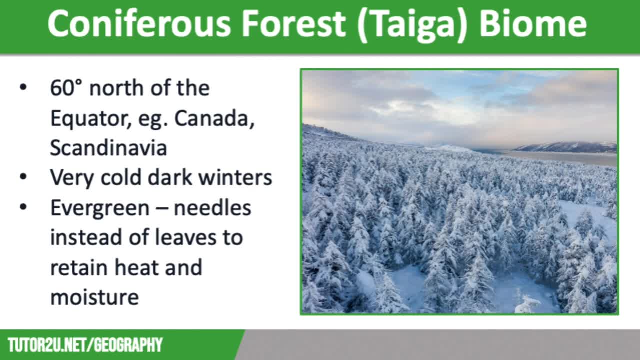 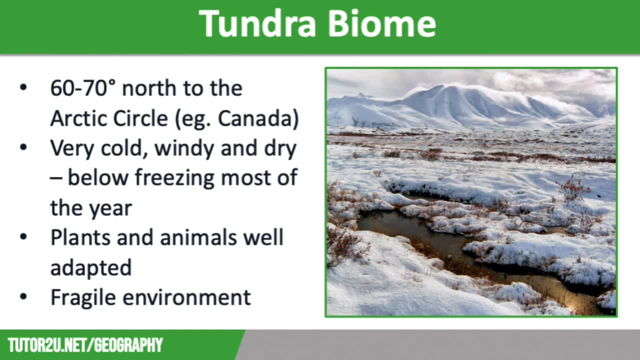 photosynthesis during the short summers. Now, moving on to a biome that many of you will have studied as part of the optional cold environments topic, This is a tundra. The tundra lies about 60 to 70 degrees north to the arctic circle, in Northern Europe and Canada. 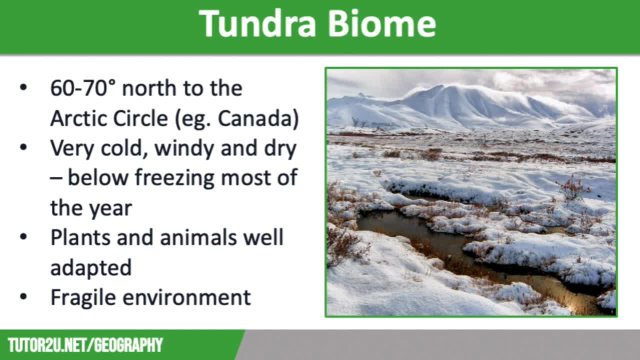 This biome experiences very high temperature and high humidity. The tundra is a very high temperature and very cold, windy and dry conditions. It's below freezing for much of the year and this is because of the angle of solar radiation, meaning the sun's rays are spread out over a large area. 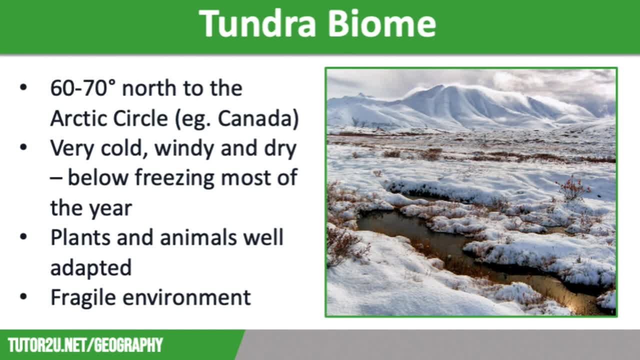 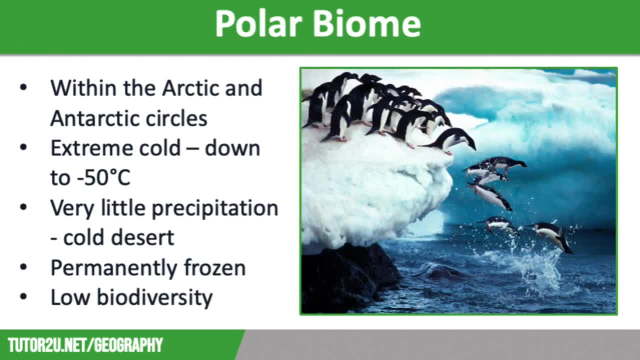 as well as tourism, And we're going to round off the video with a quick look at the coldest of all the biomes. The polar biome lies within the arctic and antarctic circles. Cold air sinks here, so the temperatures are extremely low and they can drop to minus 50 degrees. There is very little. 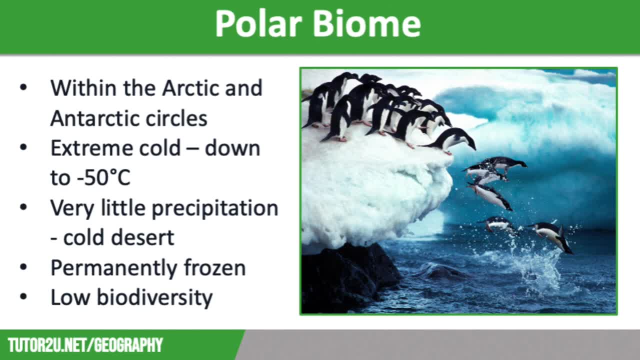 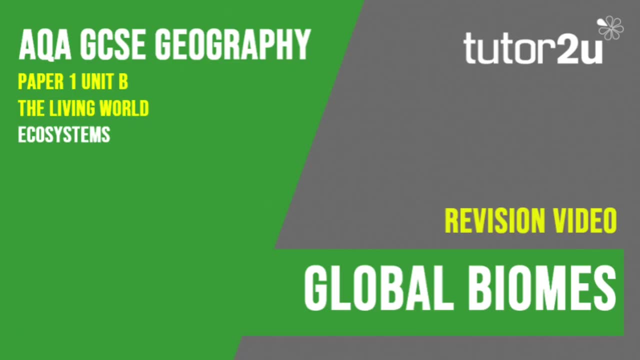 precipitation, making the poles officially deserts. The main polar regions are Antarctica and Greenland, where the land is permanently frozen and there are very few people living in the polar regions. There are very few plants and animals in this biome, as the conditions are so harsh.